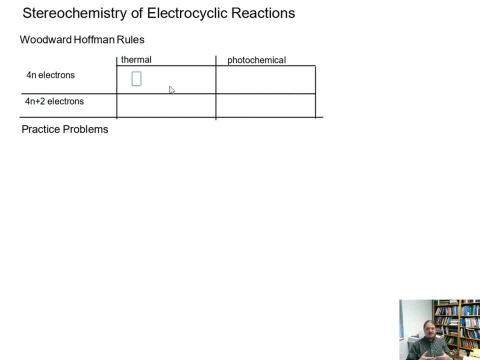 And the Woodward-Hoffman rules give us a understanding of whether the stereochemical outcome will be governed by conrotatory or disrotatory motion in the electrocyclic reaction. And so for 4n electrons with thermal using, under thermal conditions, we get conrotatory motion. 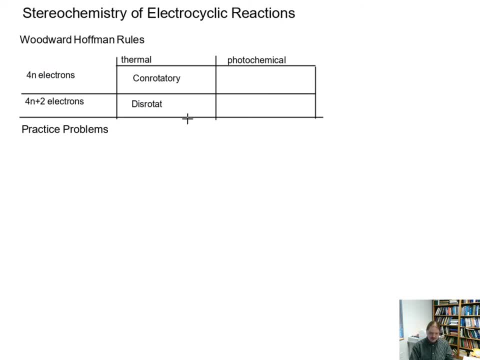 For 4n plus 2, we get disrotatory motion under thermal conditions, And then things are opposite under photochemical conditions. So here's the table. This is it. These are the Woodward-Hoffman rules, So we can use this information to help us predict the stereochemical outcome of various reactions under different conditions. 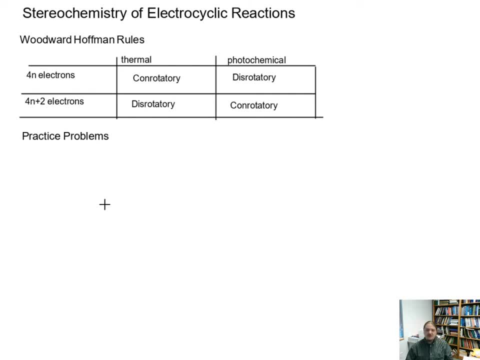 So let's do this one. Here's an electrocyclic reaction that's being done under heat, For thermal conditions, And the first thing we need to do: we know we're under thermal conditions, but we need to know whether we have 4n electrons or 4n plus 2 electrons. 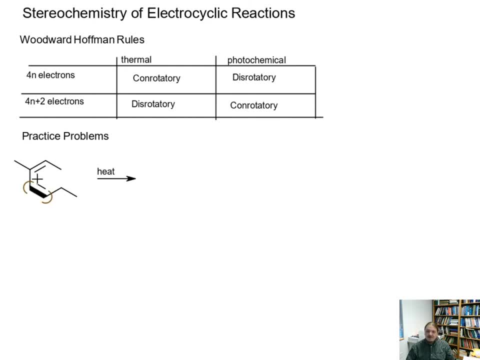 And so what we need to do, we count up the pi electrons in the pi bonds in the system, And there are two pi bonds here, Four pi electrons, That's an even number of electron pairs. So for this one, So for this one. 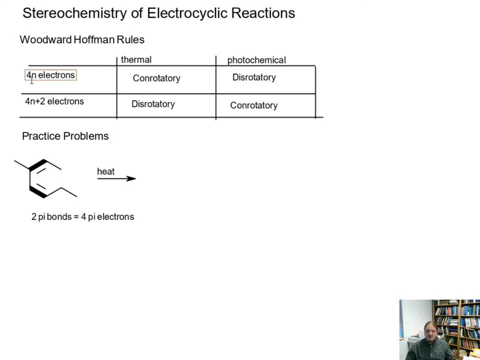 We want to go up to the table. read for 4n: electrons, thermal conditions, conrotatory motion. So that means that as the orbitals and the atoms rotate, the orbitals are rotating together, clockwise or counterclockwise. 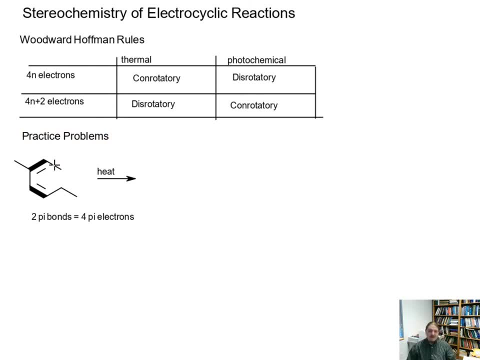 And that means that those, And that means that those, That those things, those groups that are pointing inward together, are going to rotate one up and one down away from each other. There are four electrons in the system, so we're going to get a cyclobutene. 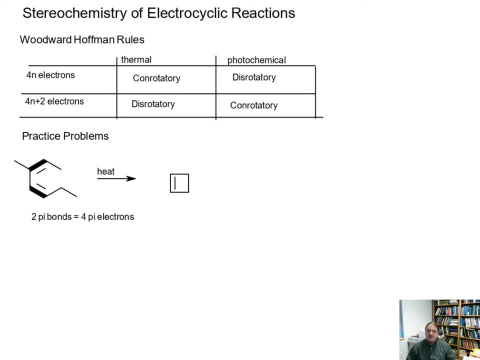 And let's say the methyl group is going to rotate down. The methyl group then rotates up And this other methyl group that's present on the other side of the molecule remains attached to the carbon atom. it's attached to, It doesn't change, and that position is planar. so we don't represent any stereochemistry there. 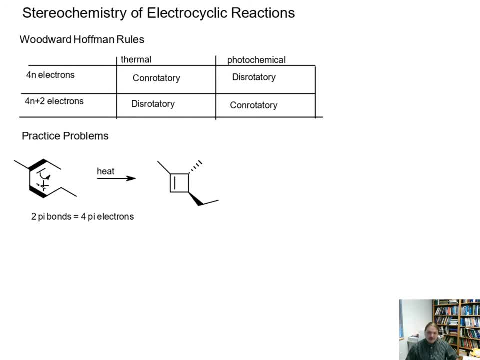 We wanted to draw the mechanism. It's a pericyclic reaction. The mechanism's pretty simple. There's our mechanism And because our reactant is a chiral, this is also going to form the other enantiomer, if we get the rotation happening in the opposite direction. 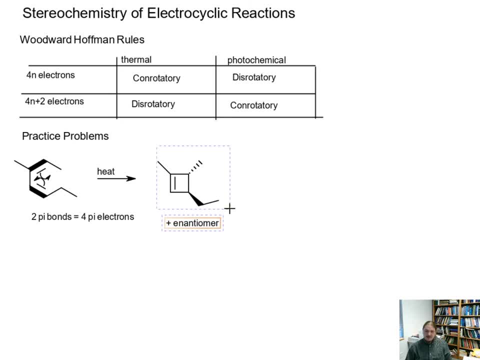 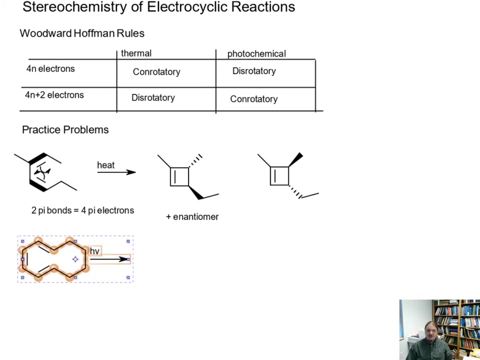 And then, just for kicks, I'll draw that other enantiomer and then we'll do another one. There it is. You get the other enantiomer when the groups rotate in the opposite direction. Here's another example. This one's done using photochemical conditions, so that HV means UV irradiation. 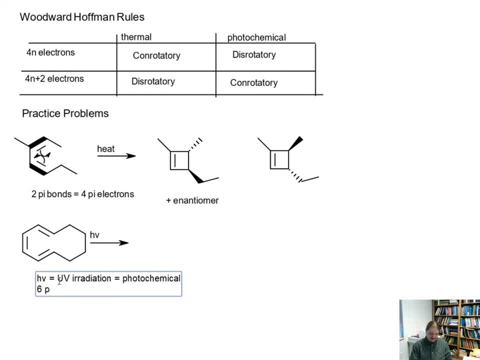 And again we have 6 pi electrons, And then we have 6 pi electrons. It's 12 total electrons. I'm sorry. No, we have 6 pi. We have- sorry, I did this wrong- 3 pi bonds, which is total of 6 pi electrons. 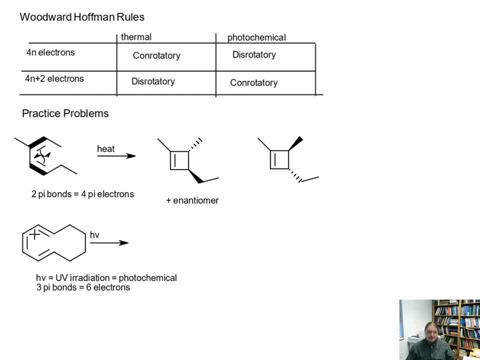 This is an odd number of electron pairs. We'll draw the mechanism And we're going to this because we're under photochemical conditions. with you know, we're going to have a lot of electrons: 4n plus 2 electrons. 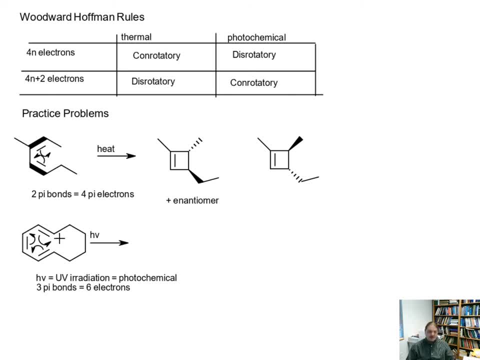 We're going to have conrotatory motion. So these things that are on the outside, one of them's going to rotate up and one of them's going to rotate down. There are hydrogen atoms in these positions. One will rotate up and one will rotate down. 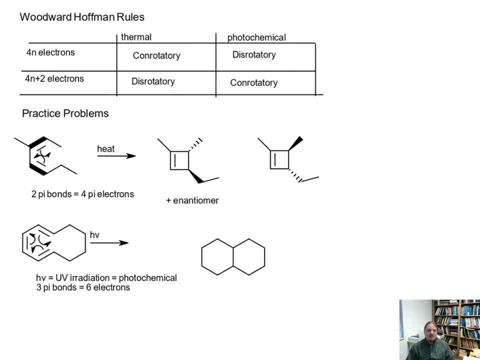 So when this ring closes together to give the decalan kind of system, here we're going to get a trans ring fusion like this And again we're going to get both enantiomers because the reactant is achiral. 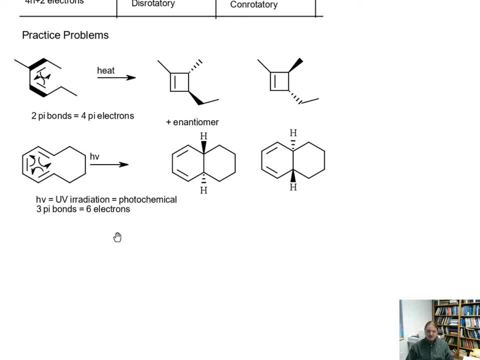 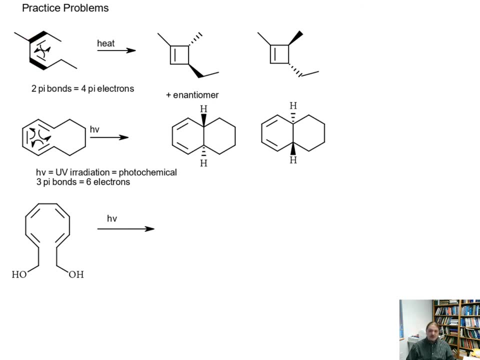 Let's do one more. This one's also under photochemical conditions. Here's a larger system. Okay, There are 4 pi, So we have 4 pi bonds here, 8 electrons And we can draw the mechanism Again. the mechanism can start at any pi bond. 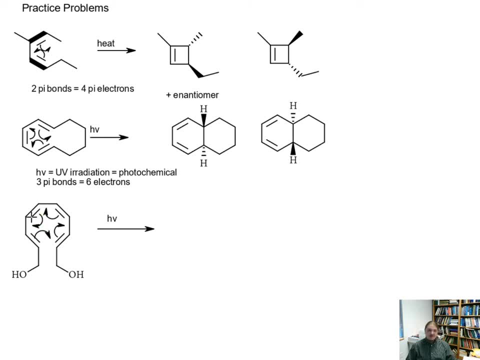 And all it needs to do is go around the circle, And it can go around the circle clockwise, or it can go around the circle counterclockwise, So you can draw the mechanism in either direction, And so this reaction's going to generate an 8-membered ring. 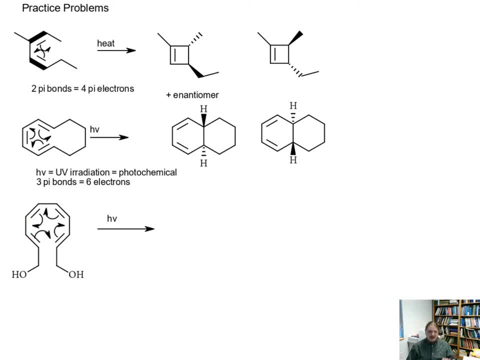 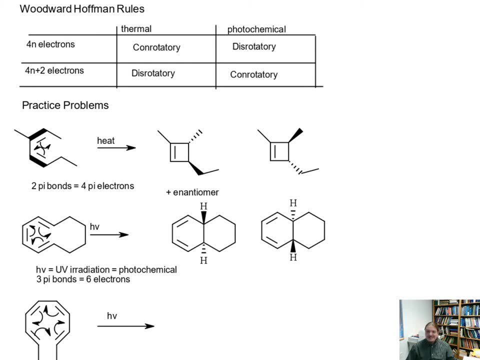 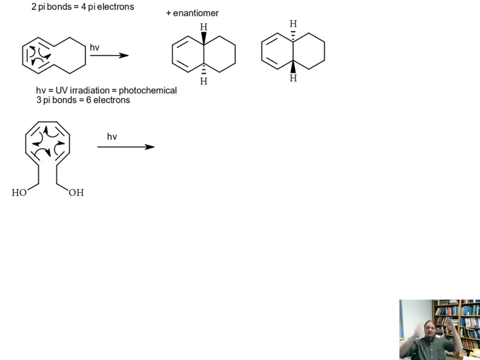 And it's got 4, 8 electrons, 4 pi bonds. So we have to go up here and look at our table. We have 4 electrons photochemical dis-rotary. So dis-rotary means that things are going to look like they're rotating together. 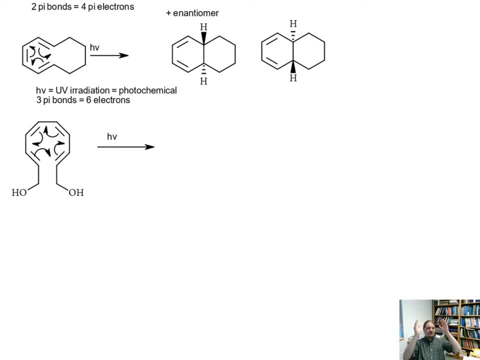 So things that are pointing in the same direction are going to continue to point in the same direction. All right. these two groups coming off of the end here, since they're both pointing in the same direction, are going to both rotate down or both rotate up. 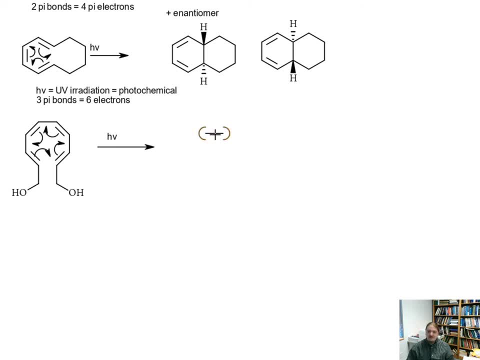 So let's get the structure of our product here. And this product molecule is not chiral. So even though I'm representing the relative orientation here, there's no enantiomer to draw. This is a mesocompound. It's also interesting to note that this reaction can be relatively 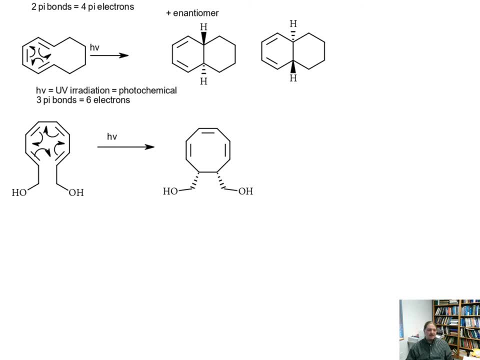 not reversible because the reactant had a. the reactant has 4 pi bonds in conjugation and the product only has 3. So it stands to reason that the reactant is more conjugated than the product. Also, I know from the confirmation of cyclooctane. 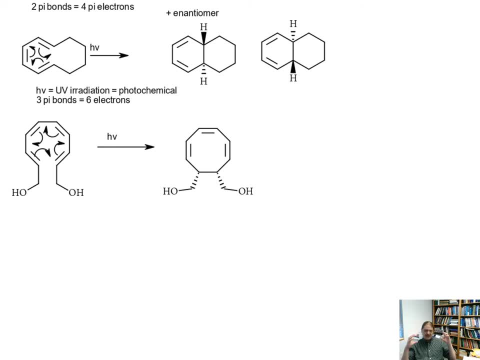 of cyclooctane or 8-membered rings with multiple pi bonds. those pi bonds are not necessarily planar, Just due to the angle stream, it would occur. So the product is significantly less conjugated than the reactant, And so you can irradiate this at something like 300 nanometers. 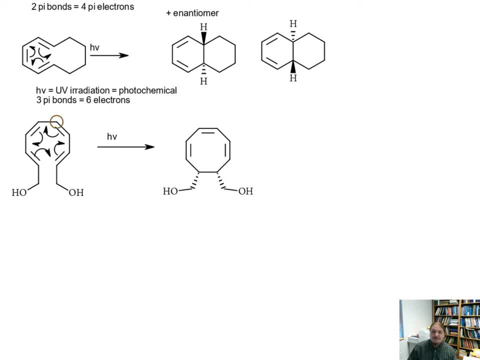 which is close to the absorbance max of the reactant And the product doesn't absorb at 300 nanometers, And you can just rely on this reaction to not be reversible under those conditions. And here's one more, And this one's also a bit more complicated. 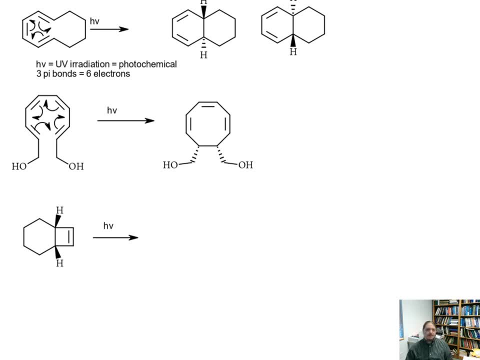 It's also under photochemical conditions, But you know, we'll do this one under heat. Well, I'll do it under thermal conditions as well, And we'll see how we get something different. Here is a reaction where I've got a cyclobutene fused. 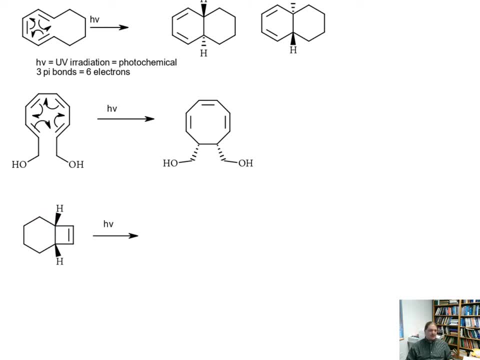 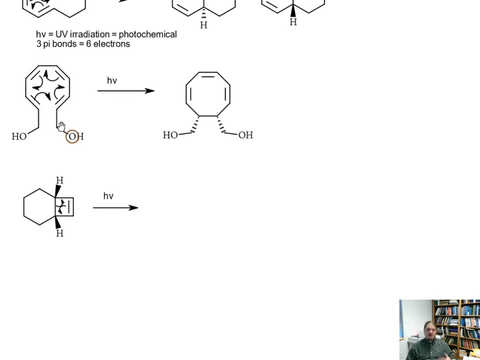 to a. cyclohexane And cyclobutenes are actually more likely to undergo electrocyclic ring opening reactions. So that's 4-membered rings And this ring is going to open and relieve a lot of that angle strain. So the question is: how do we identify how many electrons 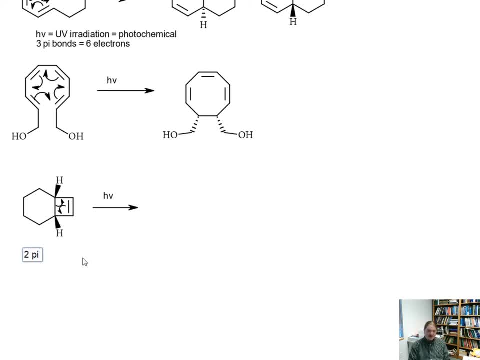 there are, so that we can go up and use the Woodward-Hoffman rules. So we have two pi electrons in the pi bond, But we're also going to have two sigma electrons that are going to count here too, And that's because, if that sigma bond breaks, 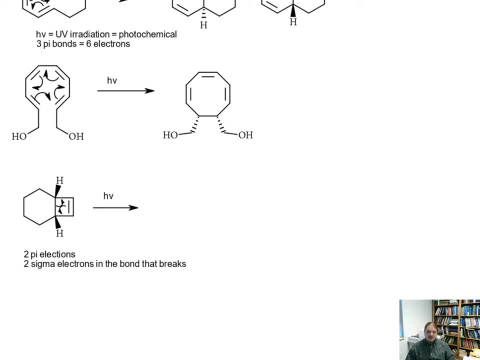 the ultimate outcome here is going to be in fact difficult to draw, depending on the stereochemical outcome, But that ring is going to open up to a 1,3-butadiene kind of system. The overall stereochemistry is yet to be seen. 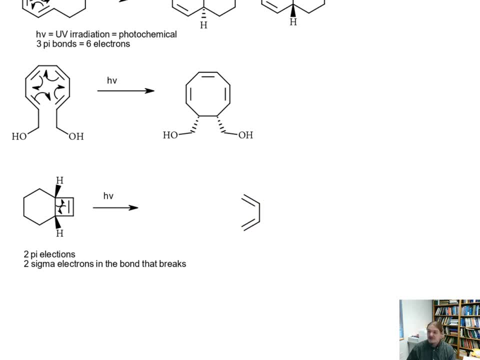 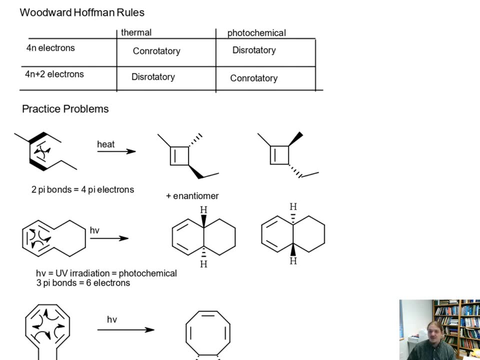 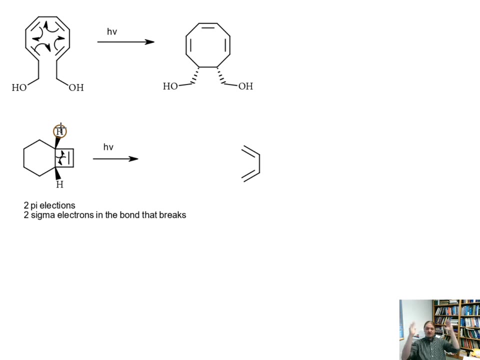 But it's going to open up here to something that has four pi electrons. So we have four electrons, So that's the first row, an even number of electron pairs under photochemical conditions. So this is disrotatory. So disrotatory means that one is going clockwise.